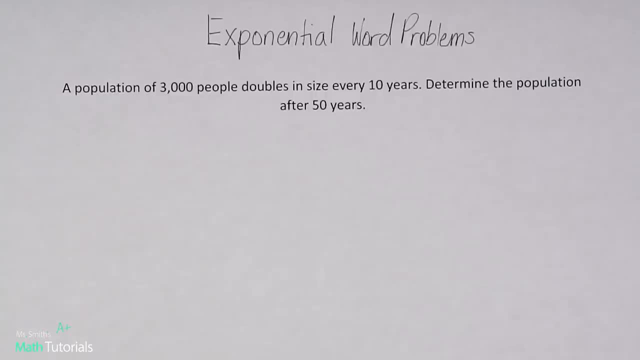 five- I believe five word problems that we're going to walk through. By the end of it you'll totally get the hang of it. They're a little weird at first, but it'll make more sense the more you do them, okay. So, starting with this first one: a population of 3,000 people. 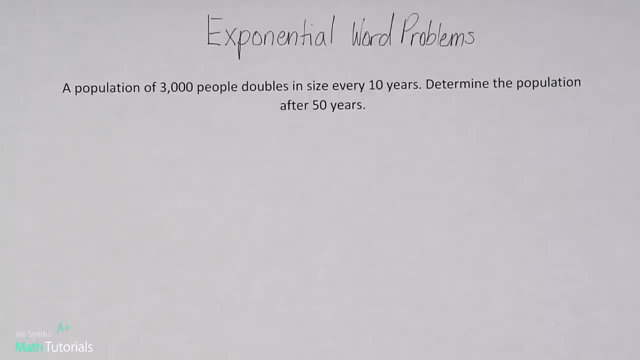 doubles in size every 10 years Determine the population after 50 years. So we're definitely this is an exponential word problem. so we're going to be using our formula: y equals n A times b to the power of x. So in my last video, you'll recall, we said a is always our. 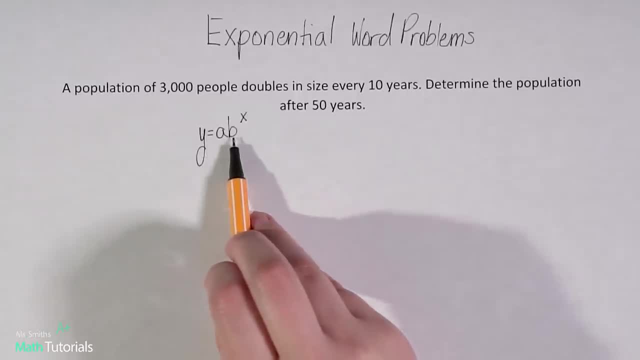 starting point, b is our rate of change and x is our time. So we need to figure out each of those three things, plug them into this formula and solve to figure out our answer. So let's start off with: I've got my y equals. a is my starting point. This is usually. 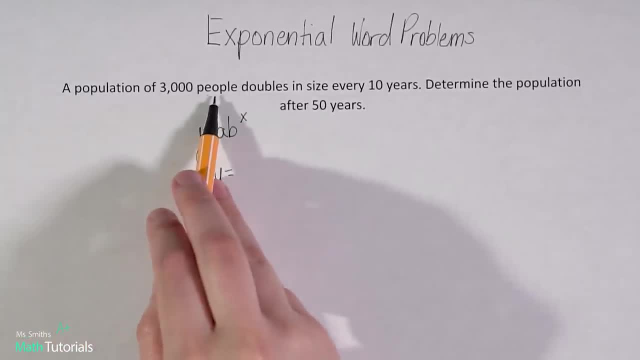 pretty clear in every problem. So it says: a population of 3,000 people. That's my starting point. So it's 3,000 is my a value? That's my starting point. All right, my b value. So it's. 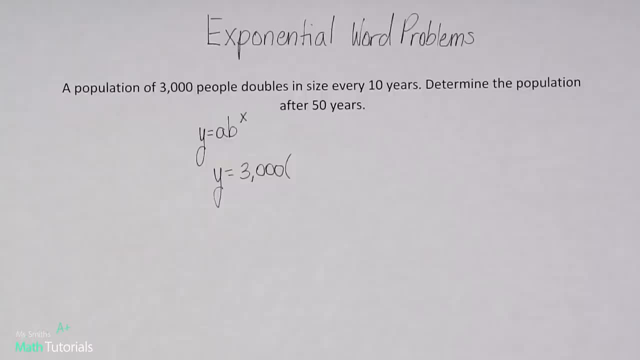 3,000 times my b. So that's going to be my rate of change. So I'll notice that this says a population of 3,000 people doubles in size. So we got to use a little bit of kind of outside the box. 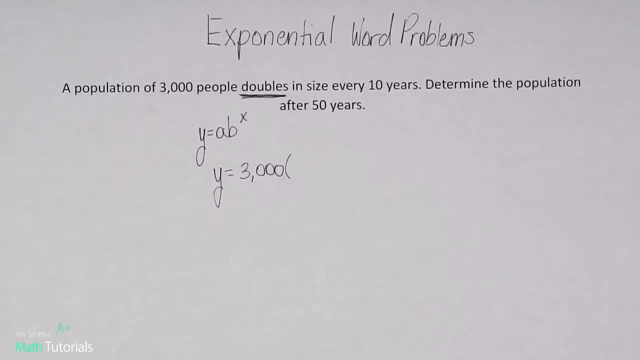 here. If something doubles in size, that means that it is being multiplied by two. Okay. in the same way, if it said it triples, that'd be times three. If it quadruples, that'd be times four and so forth. Okay, now for my x value. So it says we got to be real careful here. It's easy. 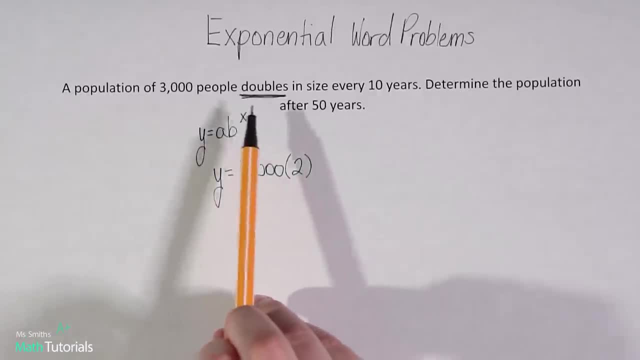 to make a mistake. This is a population of 3,000 people doubles in size every 10, years. So determine the population after 50 years. You've got to think of it. I know it's tempting to put okay, 50.. It's 50, right, Because it's 50 years. No, it doubles every 10 years. 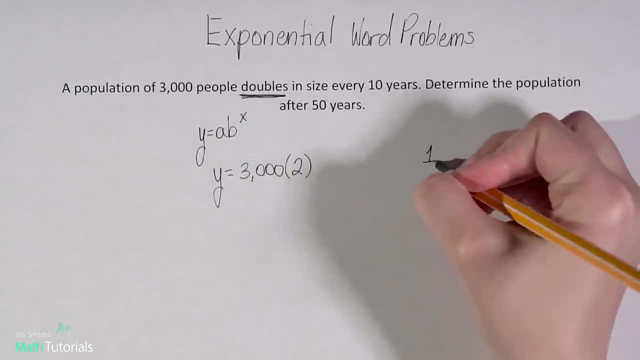 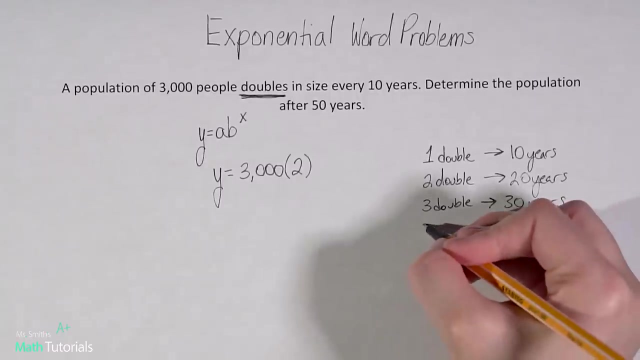 So we've got to think about: one doubling period would be 10 years, Okay. so two doubling periods would be 20 years, Alright. three doubling periods would be 30 years. So, using that same train of thought, five doubling periods would be 50 years, Okay. so what is our x? it's the number. 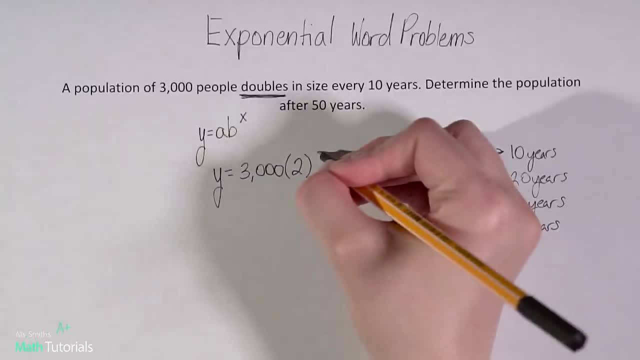 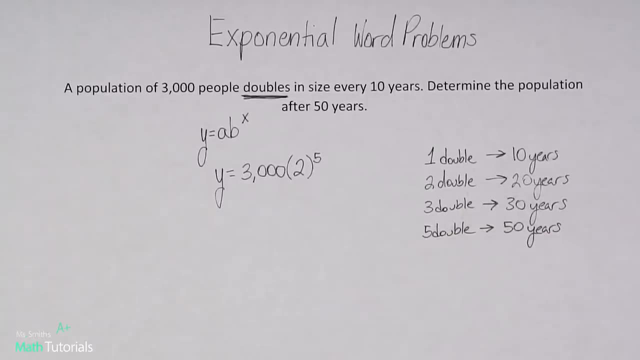 of doubling periods. So it would be five, five doubling periods. So that's kind of how I like to break it down And that's what I'll use whenever, whenever it's needed. It's not needed on every single problem, But definitely when it talks about things that double or triple or 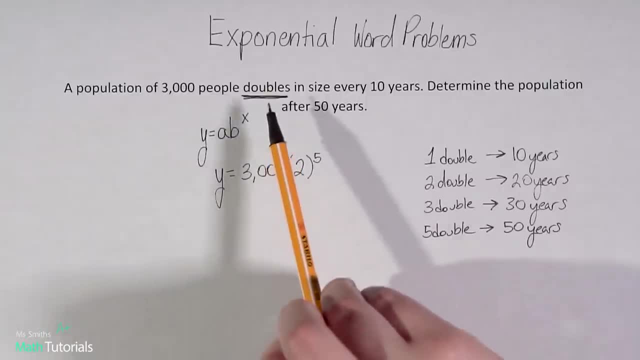 whatever increase a certain amount or decrease a certain amount every so many years And it gives you a number other than one. That's when doing this is very helpful, just to kind of lay it out, Okay. so now that I've filled in my equation, I've got my a, my b and my x value. I just put this: 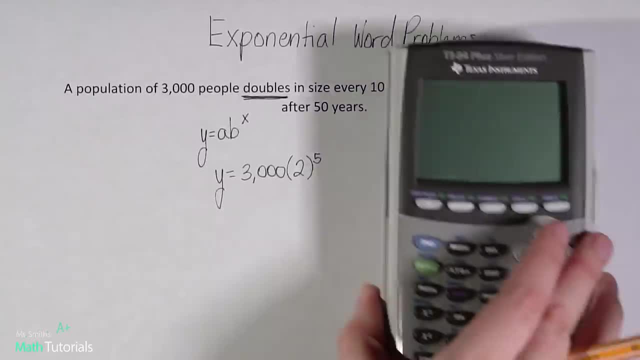 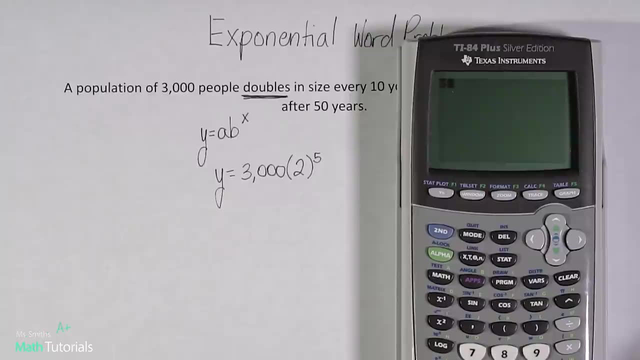 into the calculator And it does all the work for me. So I'm going to bring out my calculator, cut it on And I'm going to type this in. So 3000 times two to the power of five, It gives me y equals 96,000. 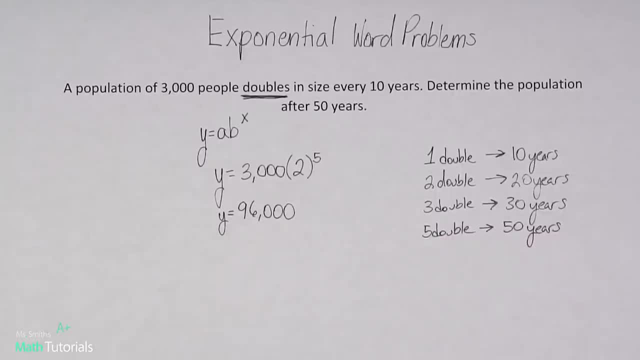 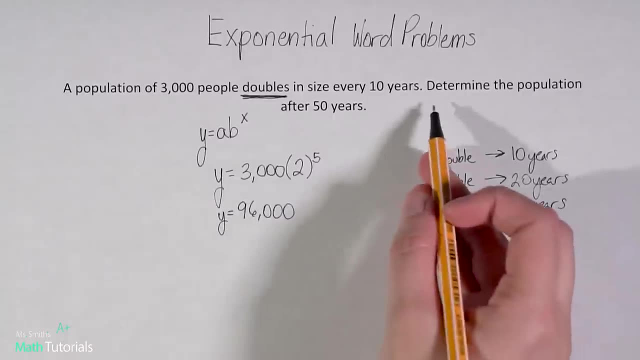 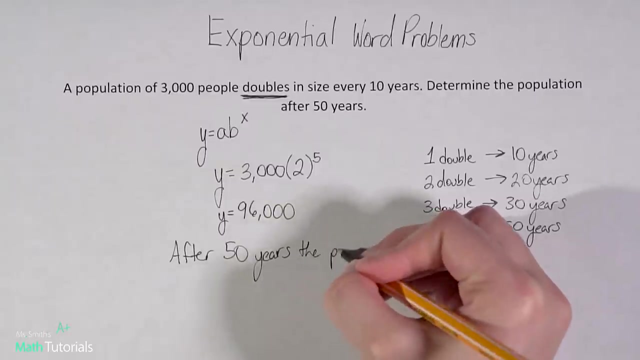 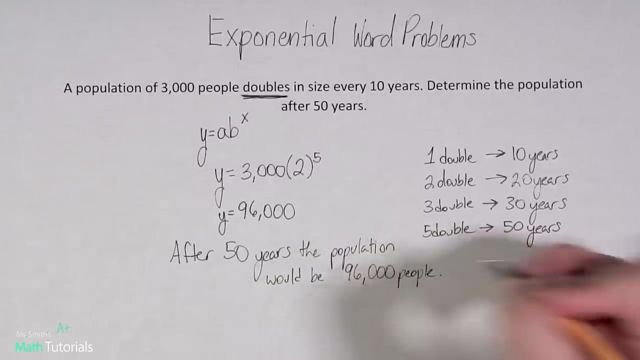 Okay, so what does this mean? Because it's important not to just have an answer, but to really state what that answer means. So the answer would be: we're determining the population. So after 50 years, the population would be 96,000 people. Okay, let's look at some more examples. 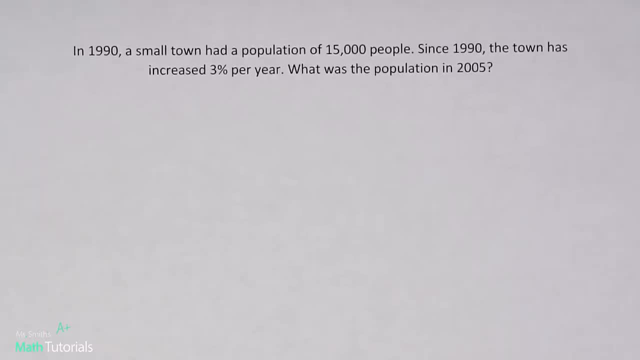 In 1990, a small town had a population of 15,000 people. Since 1990,, the town has increased three percent per year. What was the population in 2005?? Okay, so this definitely an exponential- either growth or decay In this case. we want to look for and I did not. 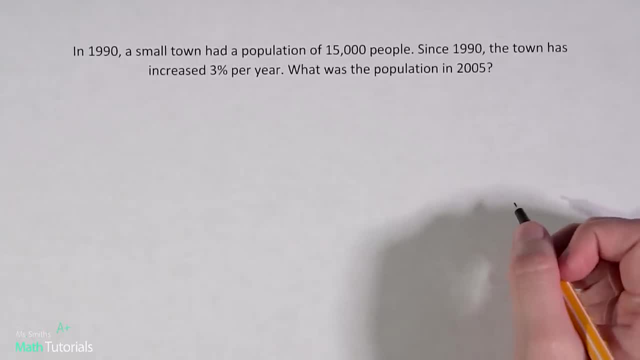 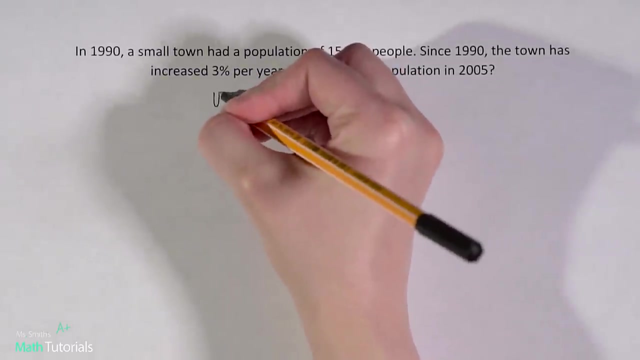 do this on the first problem, which was my bad. The first problem was a growth problem. It did double in size, so I should have noted that. So if that's helpful to you, make sure that you notice that that is a growth problem. I'll be more careful of noting that on the next ones, So I'm 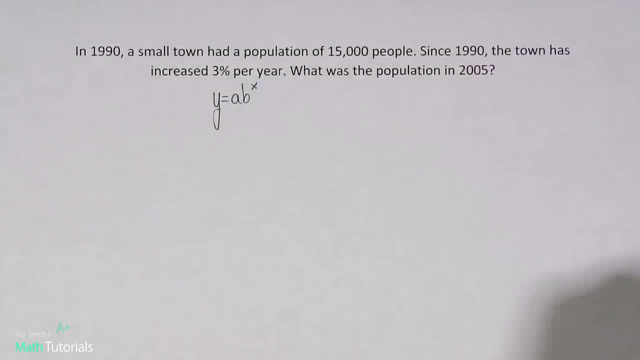 going to be using my exponential formula and I need to plug in what is my a, b and what is my x. So remember, we said a is always our starting point. So what is our starting point in this case? 15,000, right, Because we're starting this. you know, survey of sorts in 1990, and there were 15,000. 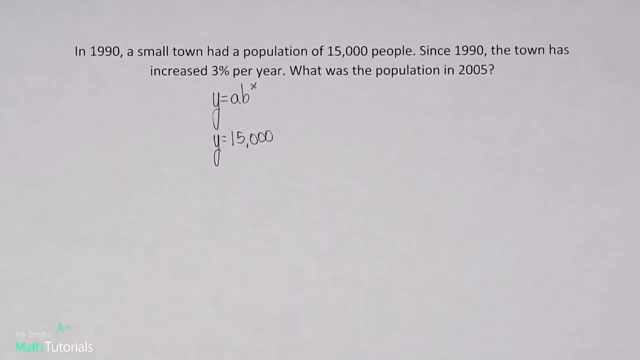 people in there at that point. Okay, now we need to look at the exponential formula. So I'm going to look at the exponential formula. So I'm going to look at the exponential formula, So I'm going to work on our b value. So our b is our rate of change. So it's increased 3%. This gets a little. 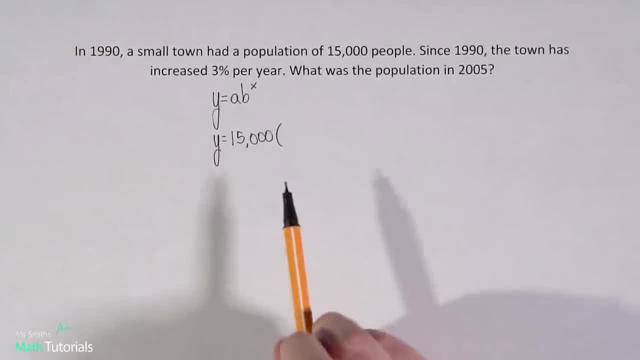 tricky. Okay, we cannot write. oops, we cannot write in for b 3%. Okay, we can't do that. Anytime it gives it to you in a percent form. there is a two-step process we have to go through. We have. 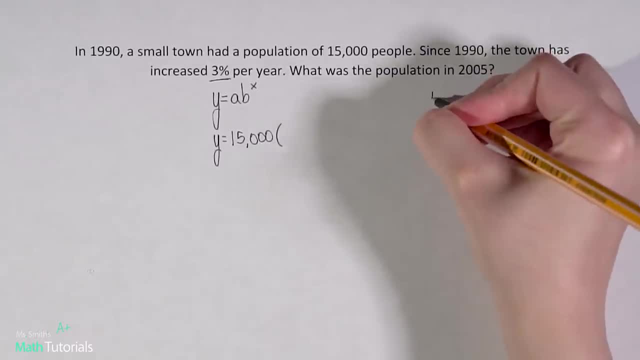 to go through all of those steps, and then we know at time, and then we'll see. So let's do it Now. first things first. let's do a column. So the column has to be passenger 1, covering number 1, and then it has to be passenger 2, sweet pesos. So you just have to do the column. 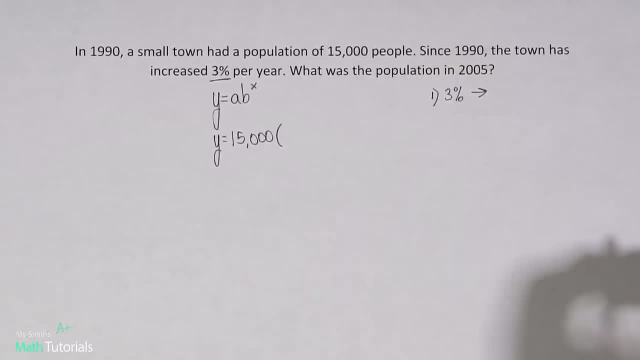 number over the number twice. Okay, now I'm going to remember the date, but we have to find the date for the demar, otherwise we do that in a fifth place, just like the first five stars. Or you can do it just like this and we have to move that После, do way back a second step, or we do. 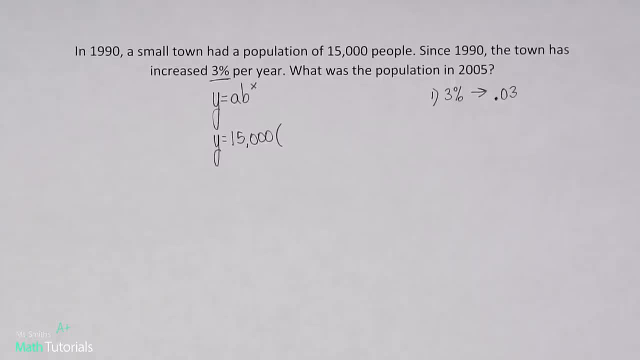 the whole together. eventually it will look like this: Now the two-step process starts with you 0.03.. That's our first step. Our second step- to get our B value when given a percent- is to ask ourselves: are we increasing or are we decreasing? Is this growth or is it decay? We had the 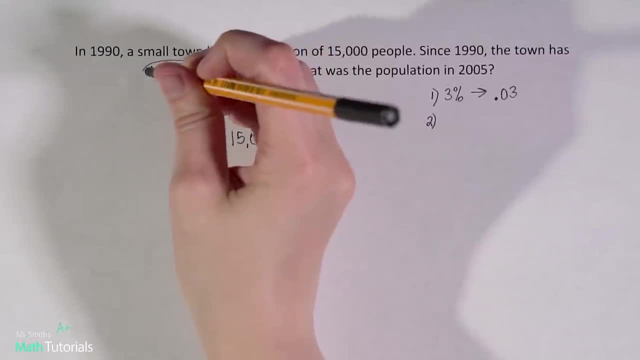 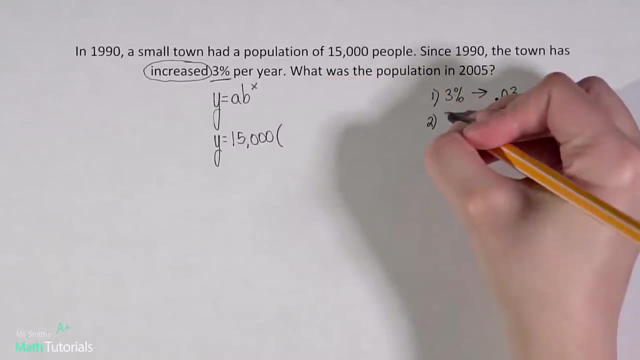 population of 15,000.. It has increased. that is a key word: increased 3%. When it increases, you do 1 plus that decimal value, 0.03.. If it was decreasing, we do 1 minus 0.03.. Don't let that. 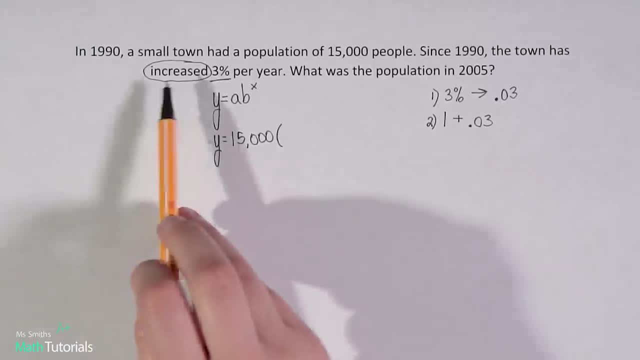 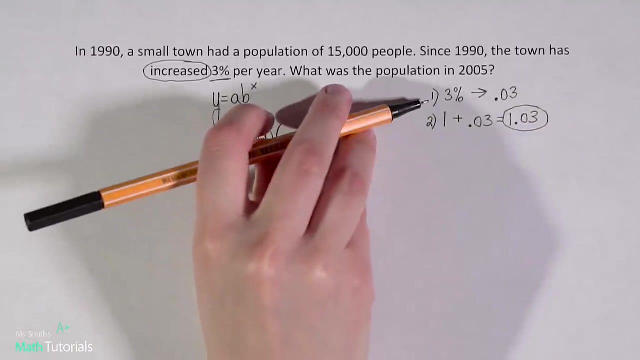 confuse you. We'll get to an example where we see that Because we're increasing, this is growth. we add the 1.. Our answer would be 1.03.. That is our B value. You've got to go through not only the first step, but the second step as well. Now we have 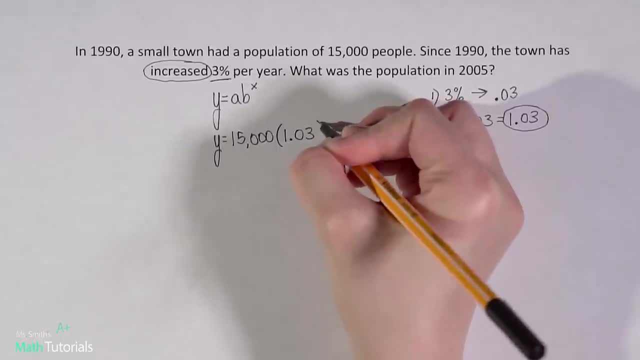 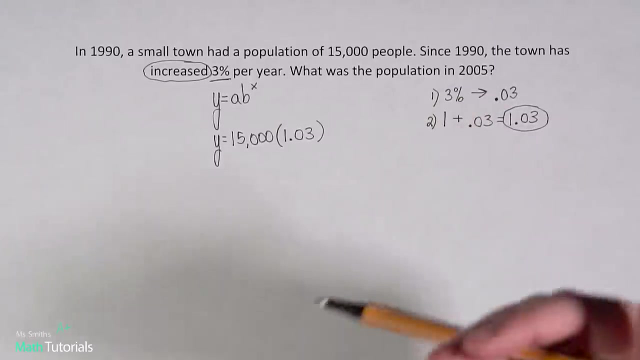 our B value, 1.03.. To the power of X. what is our time? In this case, we're talking about years. It says we're going from 2005,, but we're going all the way back to 1990.. We need. 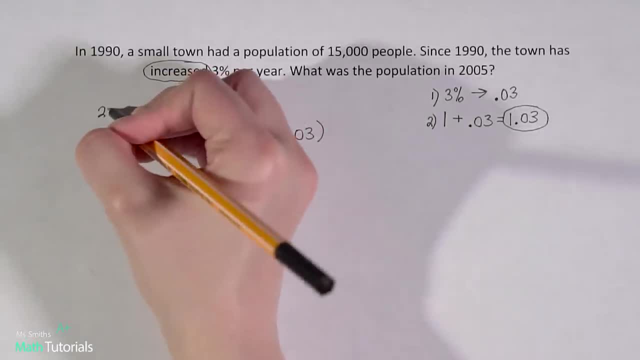 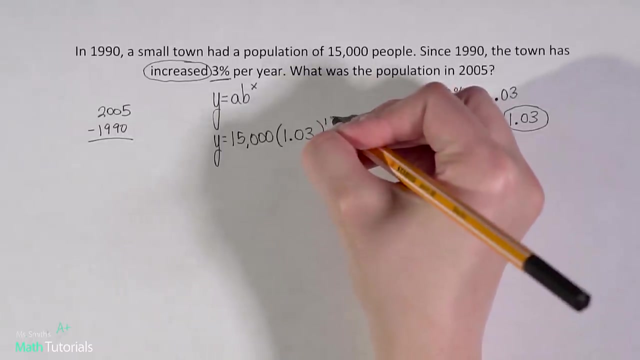 to know what is the difference in those years. You could literally do 2005 minus 0.03.. That's two thousand five. I'm going to do it on my calculator: 2,005 minus 1990.. It should be 15.. That's a 15 year difference. Now that I've got this in, I'm going put it. 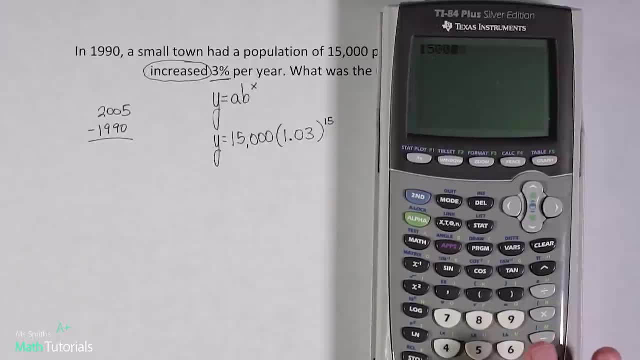 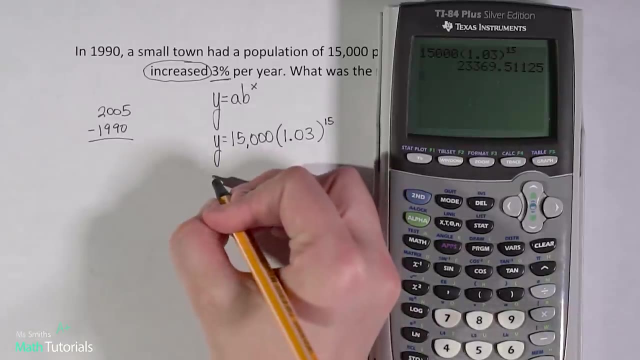 directly into my calculator: 15,000 times 1.03, to the power of 55,000.. okay, so we got to be kind of careful here. you'll notice I get a long decimal. I cannot have a decimal of a person. either it's a whole person or it's not. you know no person. okay, so we round. 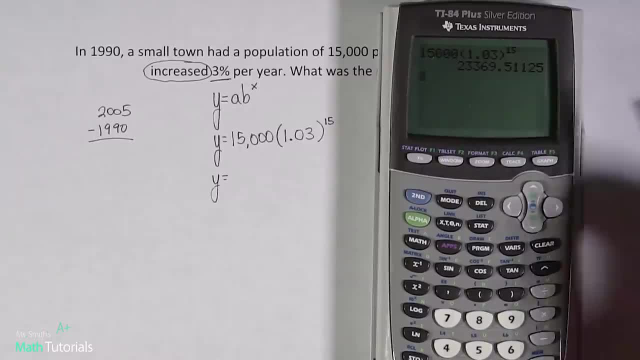 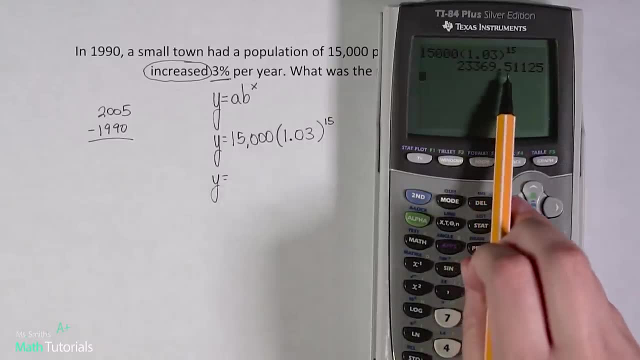 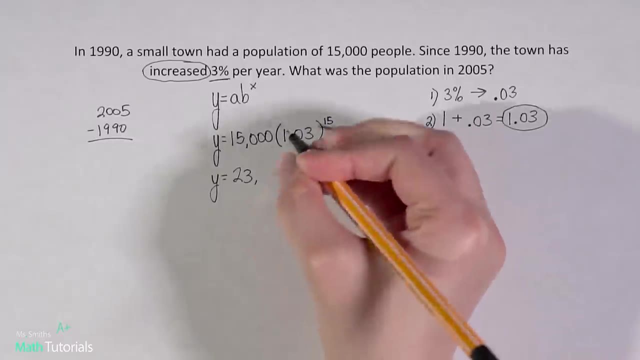 to the nearest whole number when we're talking about people, um, so in this case it'll be 23,300 and we'll round that up to 70 because of that 0.5, so it would be 23,370, okay. so what does that mean? 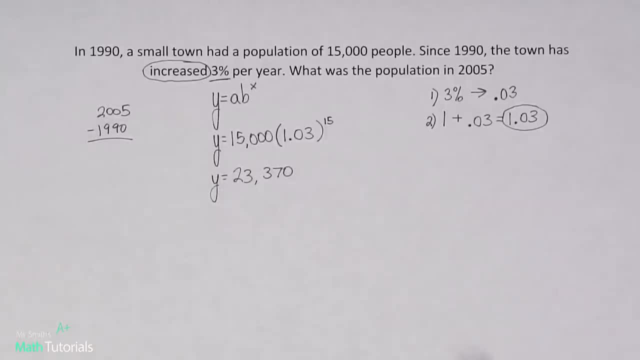 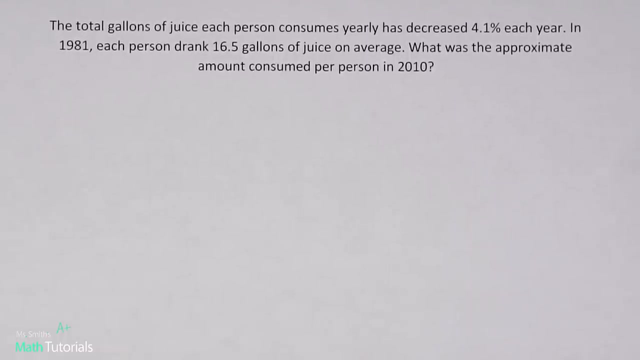 we need to take that next step and really not only just list the answer, but what does that answer mean? so in 2005 the population was 23,300 and 70 people. okay, here's another example: the total gallons of juice each person consumes yearly has decreased 4.1 percent each year. in 1981, each person drank 16.5 gallons of juice. 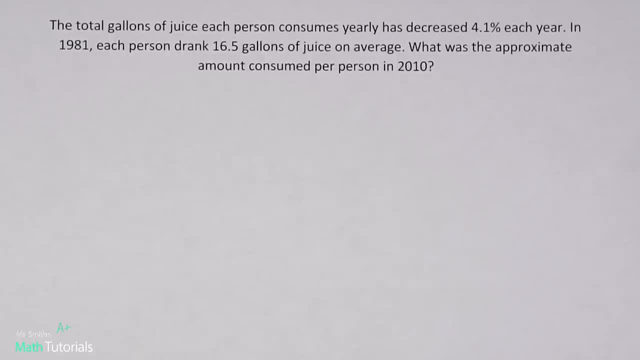 on average, what was the approximate amount consumed per person in 2010? um, so I have no idea if this is true or not- probably not, because I made it up, so, um, but let's pretend that it's true and go ahead and figure out, um what? what? the amount of juice consumed in this year was okay, so we're definitely talking about. 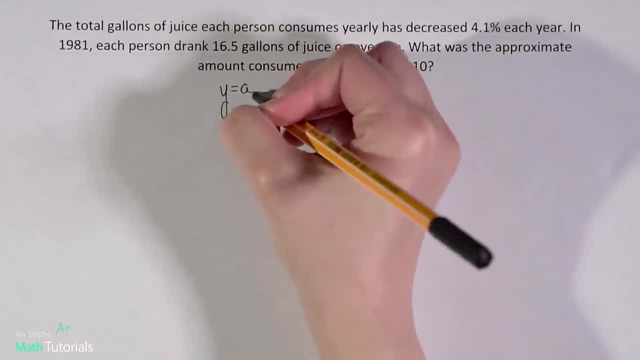 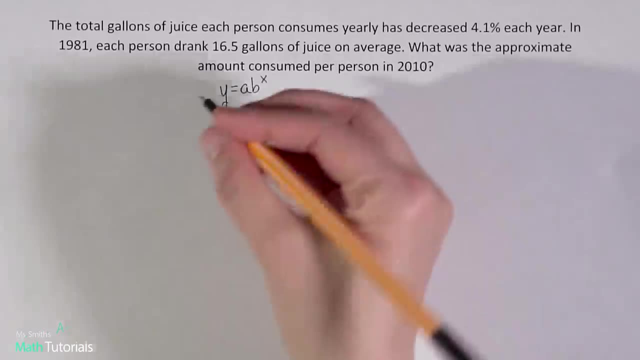 an exponential problem. so I'm going to use my exponential equation: y equals a times b to the power of x, and I just need to fill in each of those parts. so what is a? is my starting point? okay, so, for we're going to go in 1981, what was the starting amount? so it was 16.5, okay, um, so what is b? 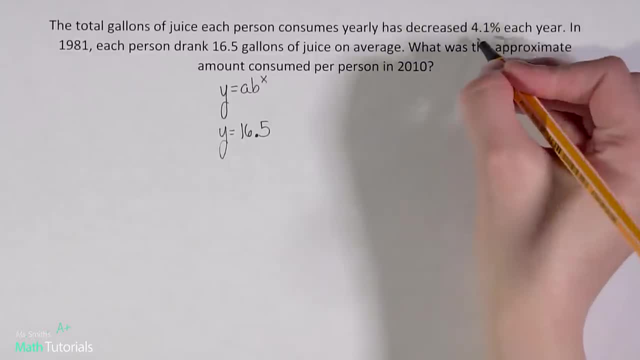 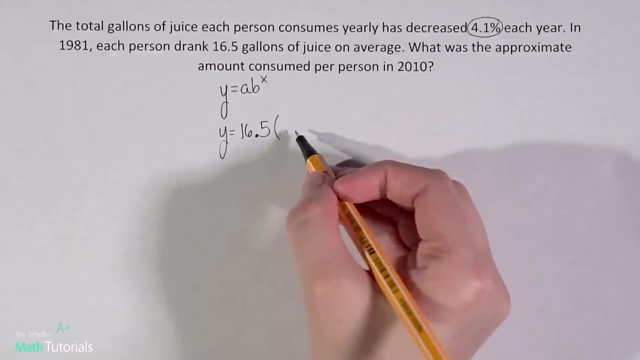 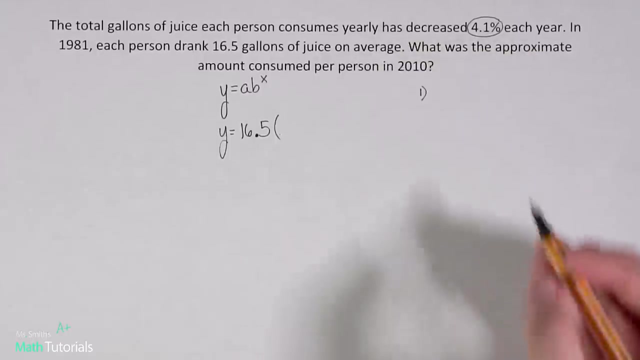 b is our rate of change. uh, so I notice that this is a percent e. so when we have a percent, I cannot just throw in here 4.1 percent. I've got to do a two-step situation. okay, step number two, step number one: turn that percent into a decimal. so whatever, your method is moving the decimal over two places. 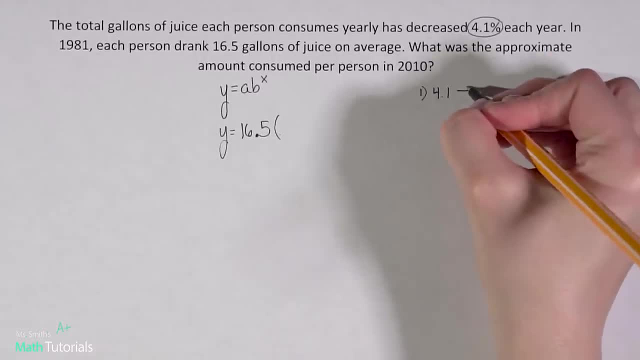 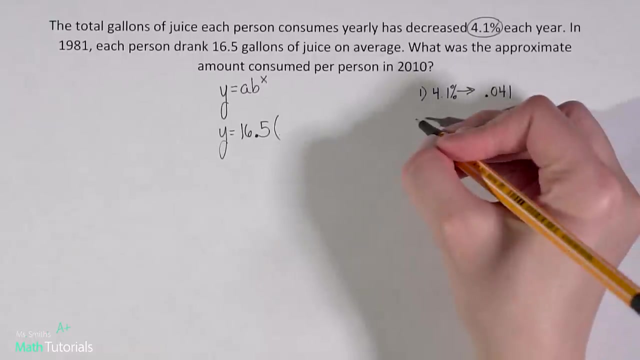 dividing by a hundred, whatever you like, 4.1 percent as a decimal would be 0.041. okay, um, can't stop there. that's not our b, yet we got to do part two. so part two says I need to take that and I need to decide: am I decreasing or am I increasing? is this growth or 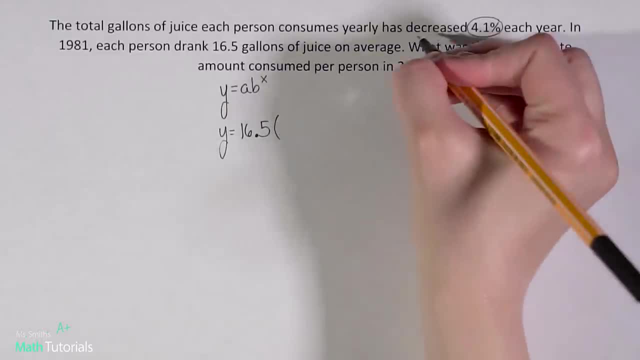 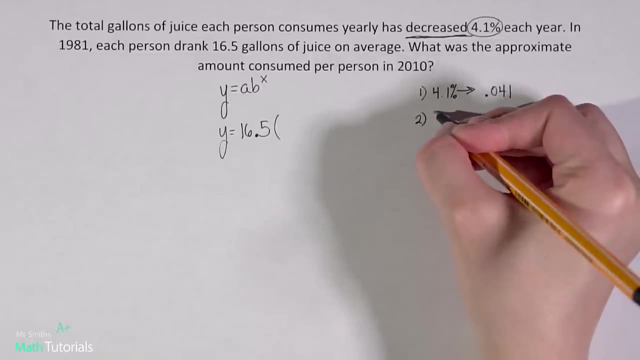 is it decay? you've got to look at your keywords in the problem, so I see that says that this is decreasing. the amount of juice people are drinking is going down, so in that case I will do one minus that decimal. okay, remember, in the last example we said: if, if we're increasing, it's a plus. 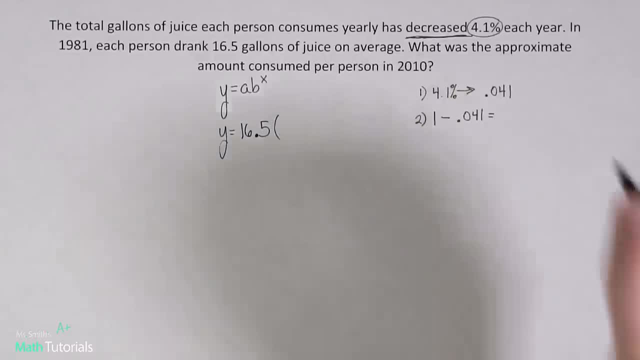 if we're decreasing, it's a minus. okay, so one- I'm gonna do that on my calculator- one minus 0.041 would be 0.959. okay, there is my b value. I went through both steps so I know I have it: 0.959 okay. 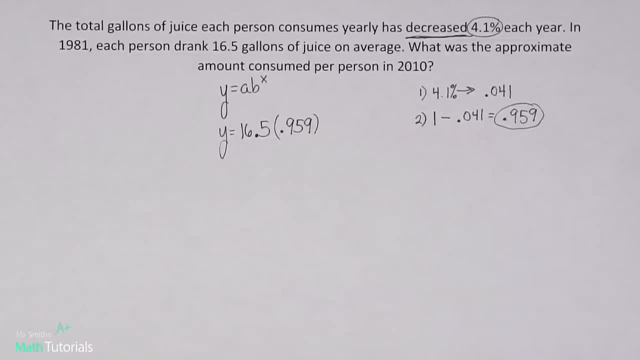 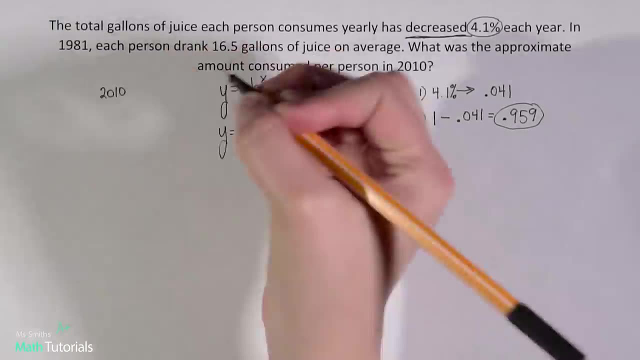 I still need my x value. we're talking about years again, like we were on the last problem, so I got to figure out what is the difference in the year. so we're going from 2010 all the way back to 1981. okay, so I want to find out my difference here. 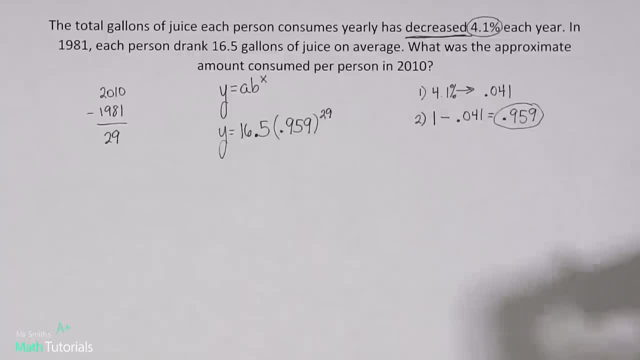 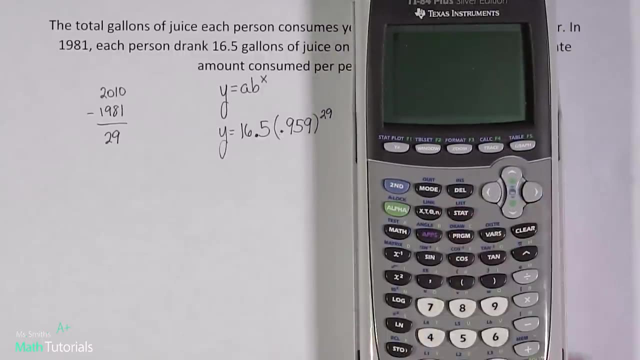 so my x value is a difference of 29 years. so now that I've got my formula, I've got each part filled in, I can just put it straight into my calculator. so 16.5 times point nine, five, nine to the power of 29.. 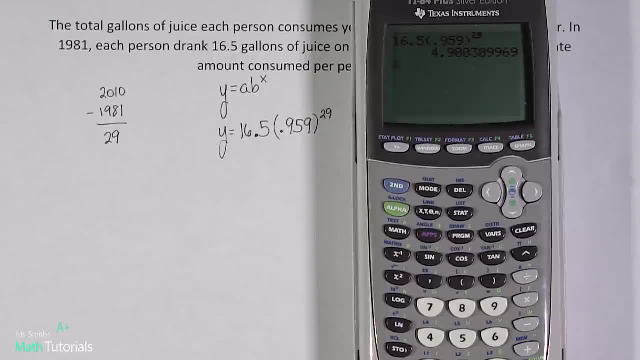 okay, now I definitely want round that decimal. I do not want to list that whole thing in my answer- and it says approximate. we're talking about gallons, so you can absolutely have you know half a gallon or a third of a gallon or you know a decimal of a gallon. we can't do that. 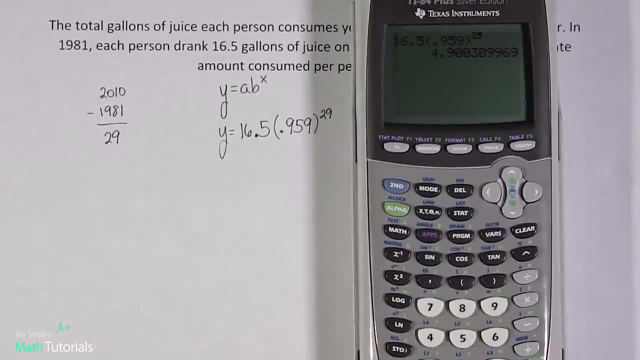 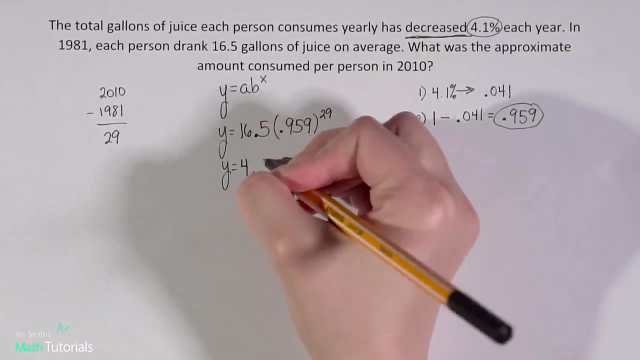 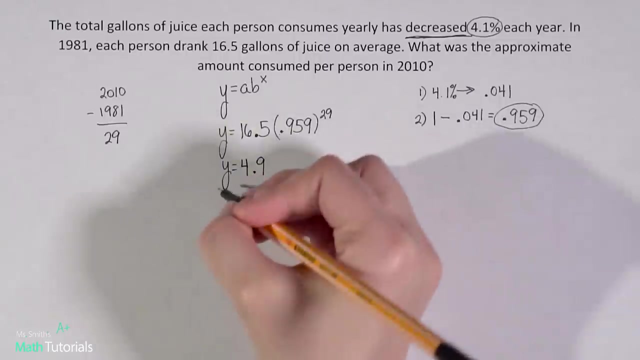 with people, but we can with things like gallons, so I'm gonna. it didn't specify in the question what to you could do: 4.9, or you could round up to 5.. Either one would be correct. I'll just stick with y equals 4.9.. Okay, so I want to write out what does that mean? So 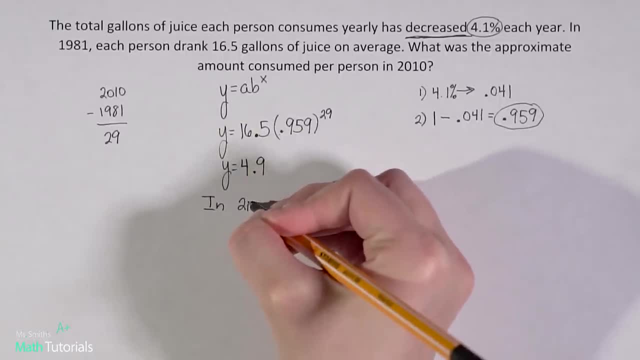 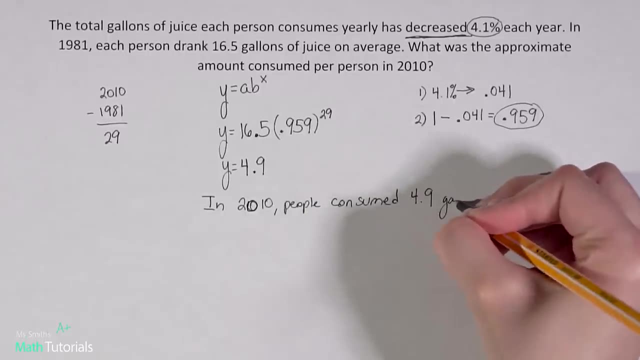 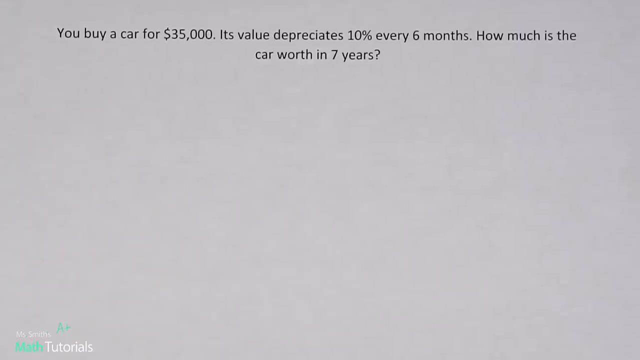 in 2010,- oops, 2010,. 4.9 gallons of juice on average. So that's per person. Here we go. Next example: You buy a car for $35,000.. Its value depreciates 10% every six months. How much is the car? 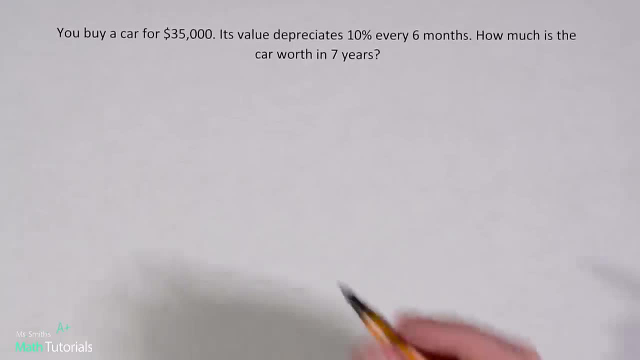 worth in seven years. Okay, so now we're talking about our exponential equation, So I'm going to be filling in. Y equals a times b to the power of x. Remember, a is our starting point. So, in this case, our starting point: how much is the car worth when you buy it? It's worth $35,000.. So that's. 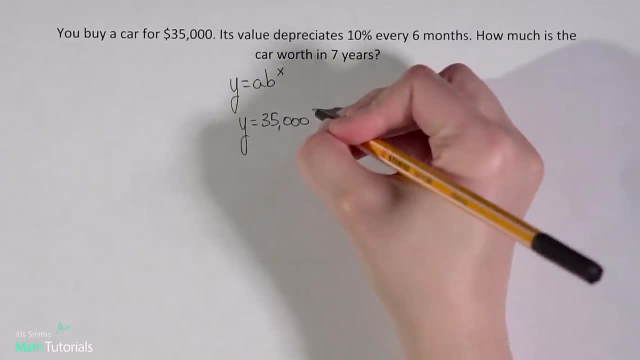 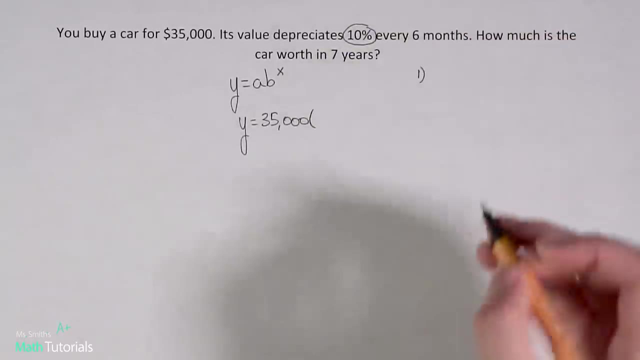 our starting point, our starting value, And then we've got to fill in our b and it gives us another percentage. So you know what that means. I've got to do a two step. Okay, first thing I got to do is turn that decimal, or turn that percent. 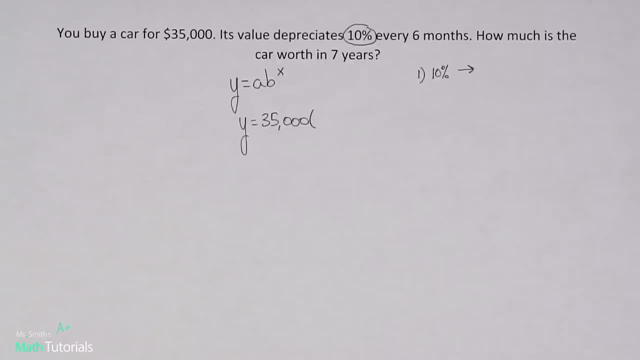 Okay, You can use your decimal trick, You can divide by 100. But however you do it, you're going to get- oops, you're going to get point one or point one, Oh, doesn't matter. Okay, now I've got to take that and do step two. I've got to ask myself: is this increasing or decreasing? 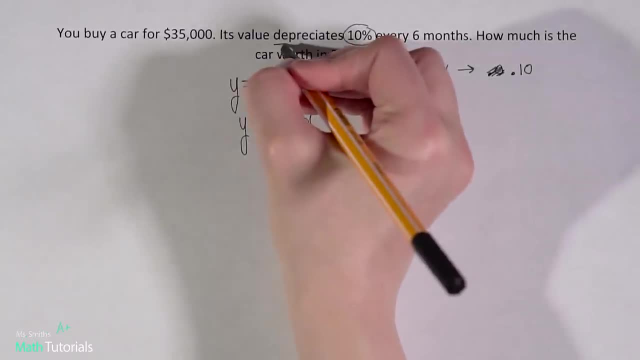 So here it doesn't actually use the word, but it does say it. It doesn't use the word decreasing, but it does say depreciates. That word means it's going down, it depreciate. So that's a word I would definitely be able to recognize: depreciates. 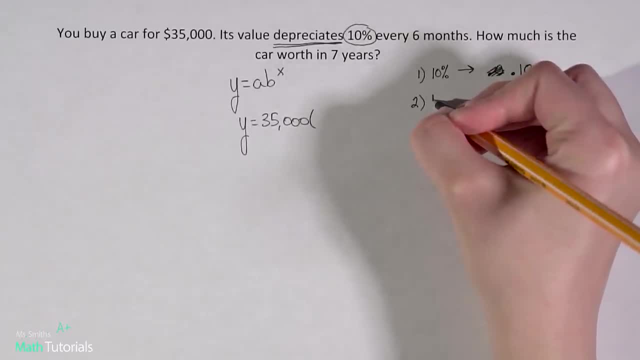 means decreases. So because we're decreasing, I'm going to do one minus that decimal. point one: Oh, okay, if it was increasing, we do plus, but it's not. So our answer here would be point nine: Oh, okay, or just 0.9.. That is our B value. okay, Got to do both steps All right. now our time here. 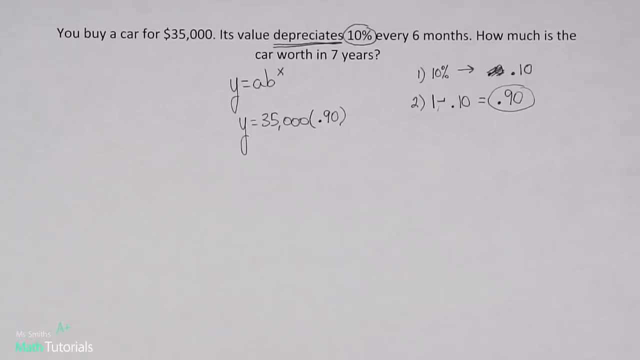 we've got to be very careful. It's easy to make a mistake here. It says the value depreciates every six months. How much is the car worth in seven years? So I know it's so tempting to just skip- and I almost did just a second ago skip and write seven, but that's not accurate okay. 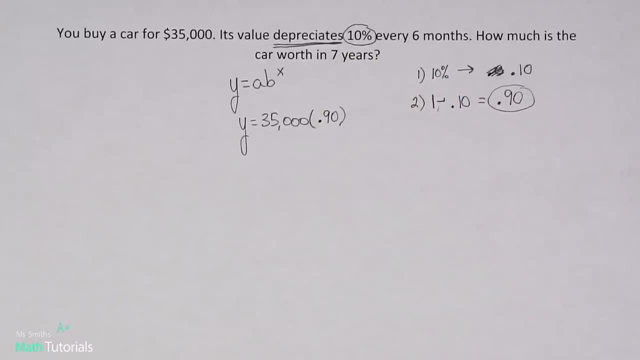 Because it's 10% every six months, not every year. So we've got to think about this, like one year would be how many cycles, how many periods of this decrease of 10%? Well, it would be two, right, Because there's six months in every year, So that would be two. 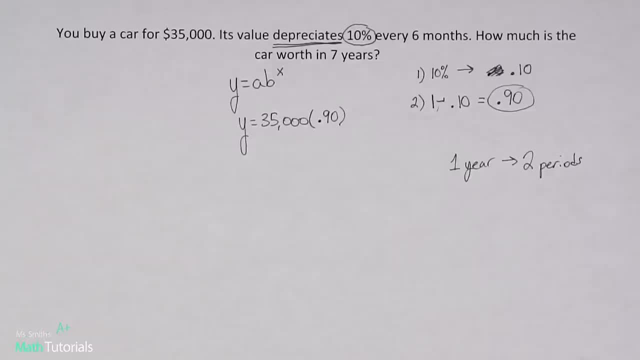 periods- we'll call it okay- of decreasing 10%. So in that case, two years would be how many periods? Well, that would be four periods. All right. what if I said four years? How many six months periods would that be? Well, that would be eight periods. 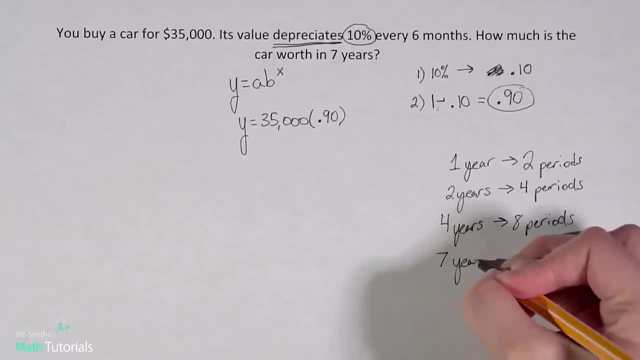 Okay, so let's think about seven. Keeping this pattern going seven years would be how many periods? Well, it'd be 14.. I'm just kind of multiplying because I know it's two periods per one year And if you struggle with making that jump, going from two to four and from four to seven, 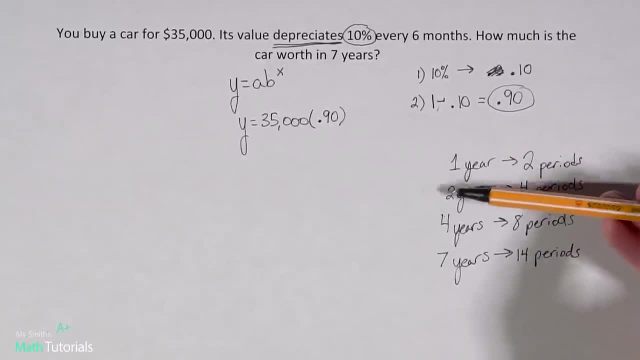 then don't make the jump. Lay it out: Do. one year would be this many. two year would be this many. three year would be this many. Lay it out all the way to seven, if that's what you need to do, okay. 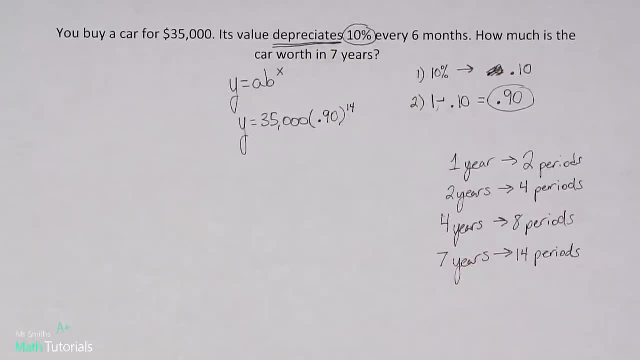 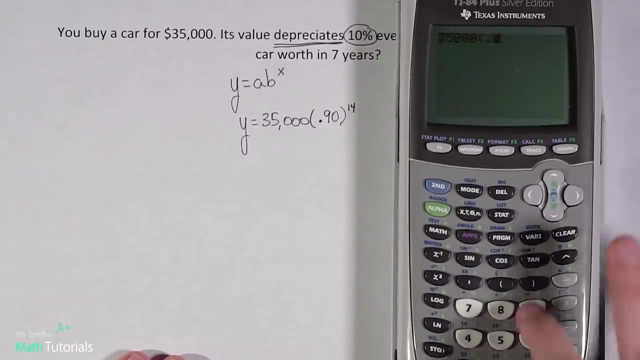 But either way it's 14 periods of the 10% increase. So really important to note that. All right, now that I've got my formula laid out, I'm just going to put it right in the calculator: 35,000 times 0.90 to the power of 14.. 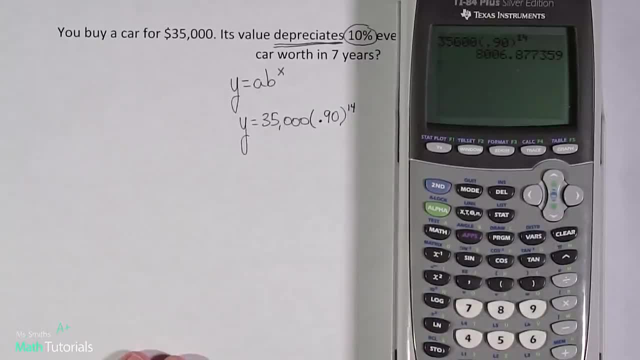 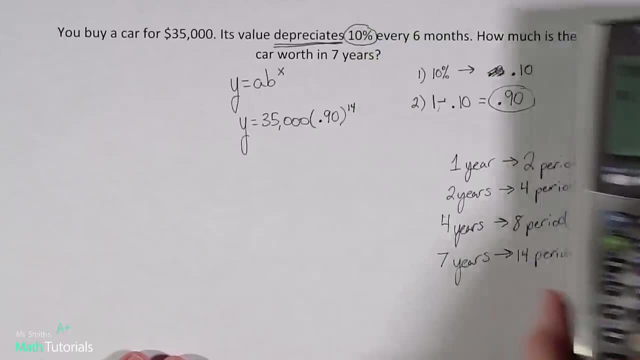 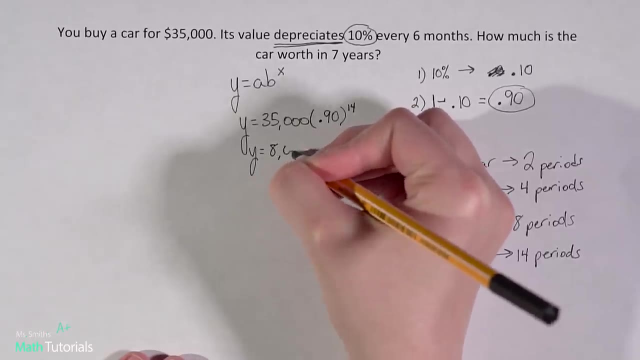 Okay, so my Y is- and we're talking about money- You could either round to the nearest dollar or round to the nearest cents. I'll do cents just because we'll be exact. Okay, so it's $8,006.88.. 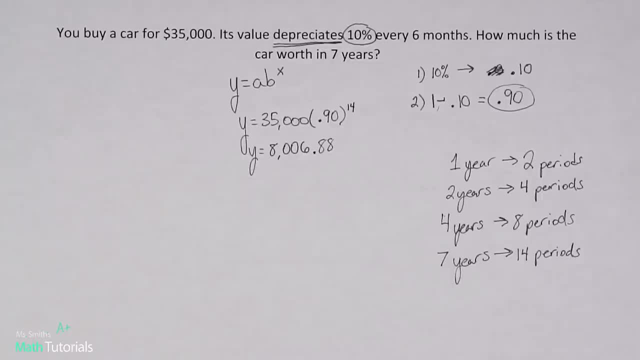 Okay so let's let's um. sorry, this is gross. Okay so let's talk about what that answer means. So after seven, after seven years, the car is worth? car is worth really only $8,006.88.. 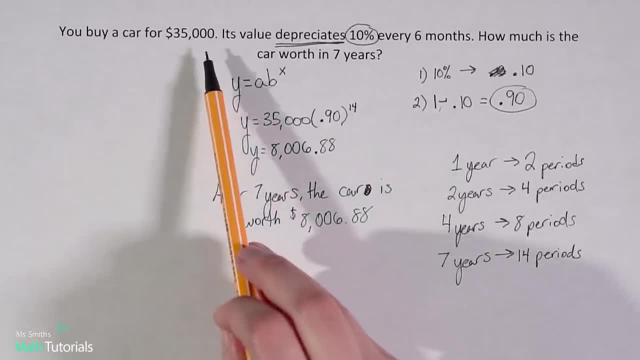 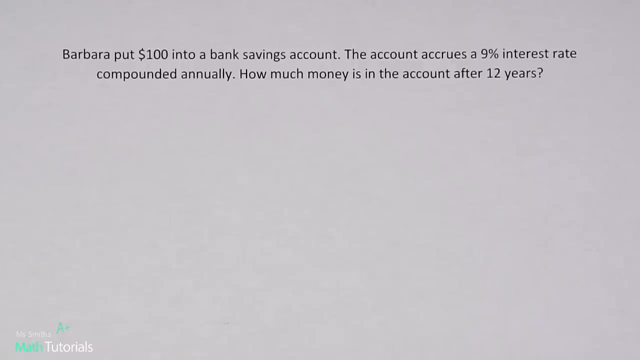 Okay, think about that. You bought the car, you spent $35,000 on it. after seven years It's only worth eight, approximately $8,000.. Um, so kind of the tough thing about owning cars. All right, we've got our last word. problem here: 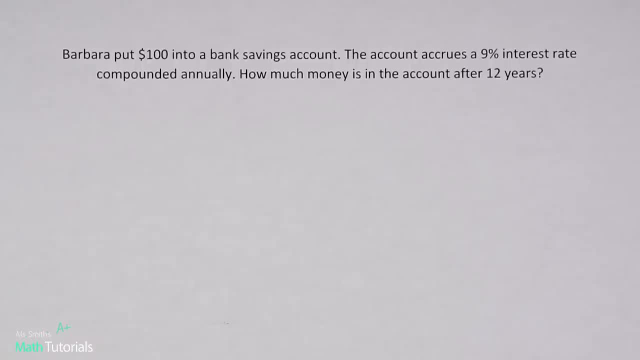 Last one, All right. so Barbara puts $100 into a bank savings account. The account accrues a 9% interest rate compounded annually. How much money is in the account after 12 years? Okay, so anytime we're talking about money and interest rates. 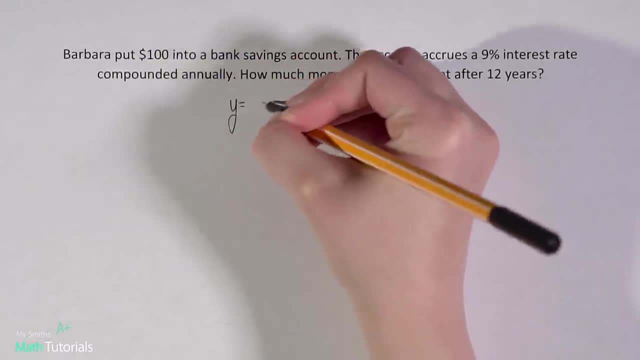 and things like that. you're definitely gonna be using your exponential growth um slash decay formula, okay, Um, so we just need to fill in each part of this. A will always be my starting point. So how much money did she put in the bank account from the get-go? 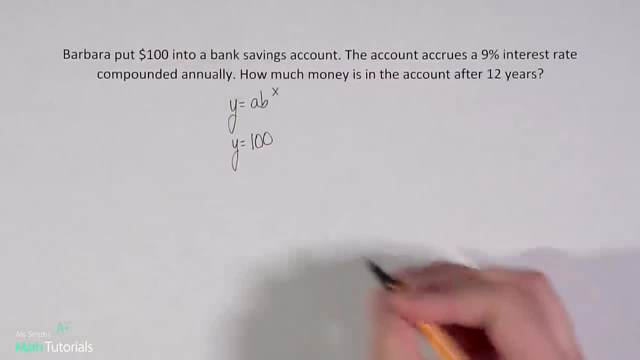 She put in $100.. So that's our starting point. Now I need my B value. Um, again, they love giving us those percents, So we've gotta get used to doing our two-step to turn that percent into an actual B value that we can use. 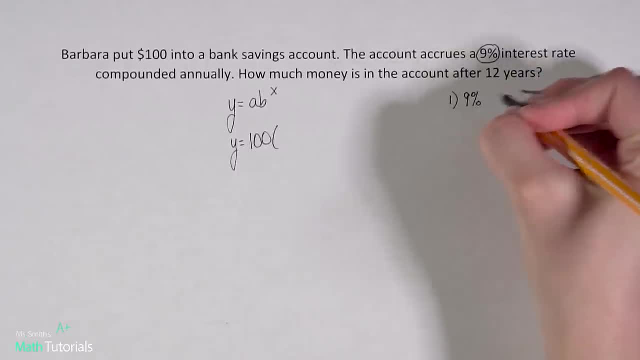 All right, first step: Turn that percent into a decimal. So, whatever method you wanna use, you should get .09, okay. Step two: Take that and decide: Are we increasing or are we decreasing? Now I know this, ninth graders um. 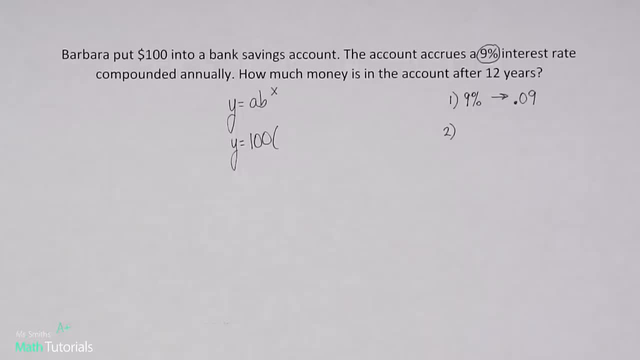 are not really used to learning about interest rates yet You know it kinda comes when you get older. So pretty much anytime you're talking about, you know putting money in a savings account and interest rates- your money is increasing okay. 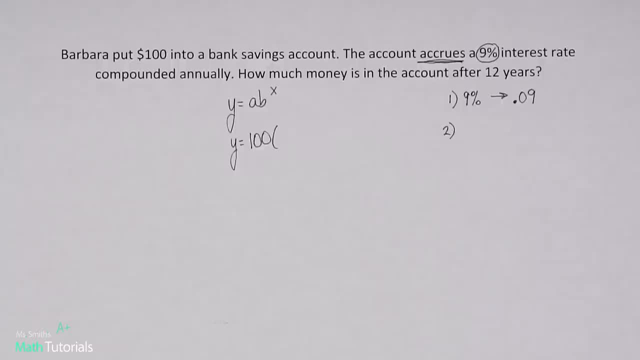 And that word accrues, that means it gains. okay, So over time it will accrue. It will gain this amount of interest compounded annually. That's a phrase you're gonna see a lot of times. You're gonna see a lot interest rate compounded annually. 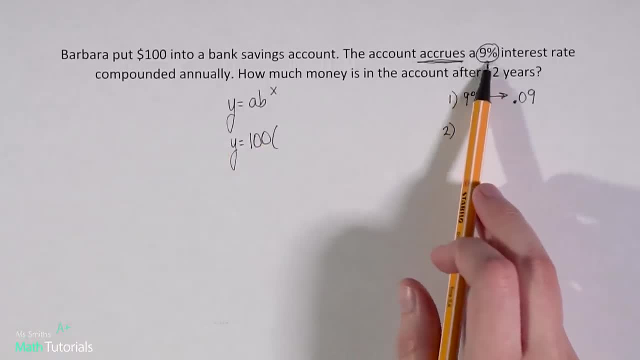 All that means is that you would get this percent of your money back in interest, gained in interest, once a year. So throughout the year you should get 9% of your money given to you as kind of a bonus for keeping your money with that particular bank. 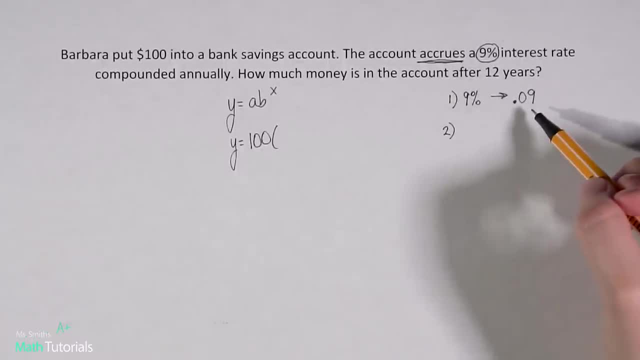 Okay, so just kind of some side information there, But the fact that it's accruing, accruing means it is going up. So we would do one plus because we're increasing that decimal .09.. So that's gonna give us 1.09.. 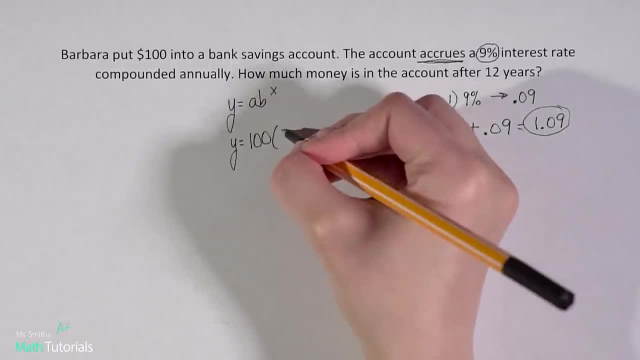 There's our B value. That's what I can use, So 1.09.. All right, now my X, my time, this one I really like. it's super easy. It's compounded annually, So it's once a year. 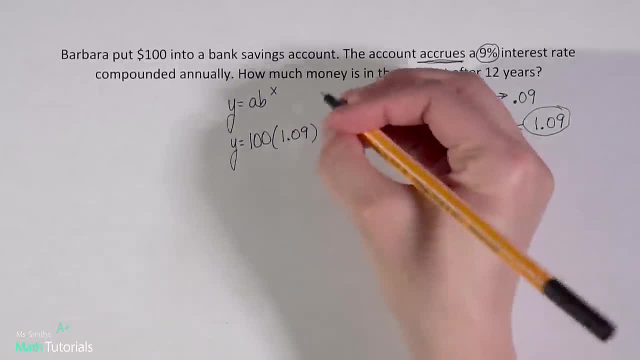 And we wanna know how much is in there after 12 years. So 12 would be our X. I like those when it's just nice and simple. We don't have to worry about doubling periods or anything like that. Okay, so now that I've got my formula all filled out. 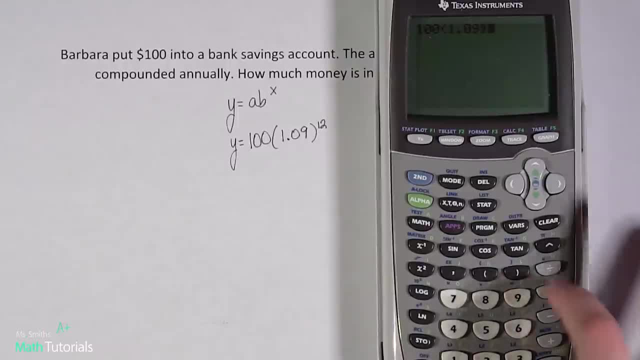 I'm gonna put it in the calculator: 100 times 1.09 to the power of 12.. All right, now we're talking about money again, So you can either round to the nearest dollar or to the nearest cents. I'm gonna do cents in this case.